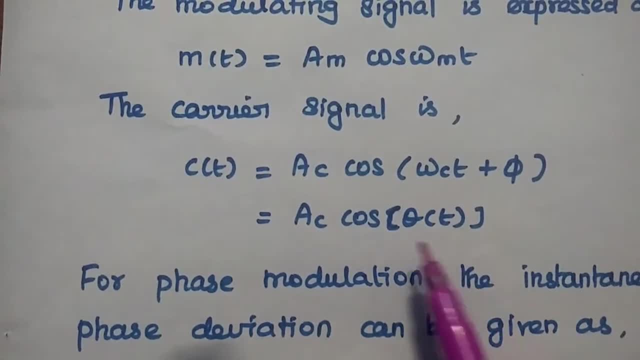 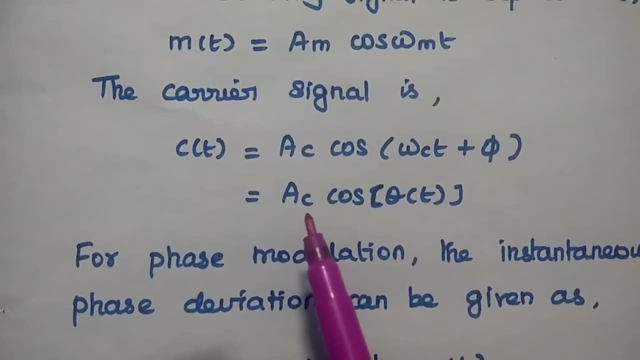 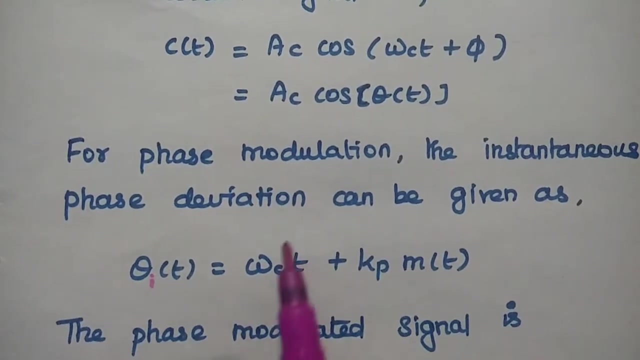 So here theta of t is the angle of the signal which depends on the phase value. a, c is the maximum amplitude. So this can be written as a c cos of theta of the carrier signal For phase modulation. the instantaneous phase deviation can be given like this: 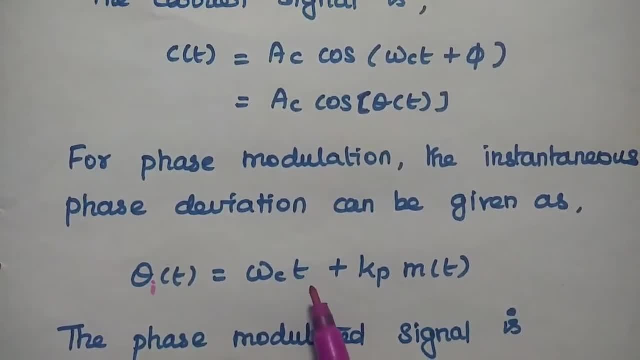 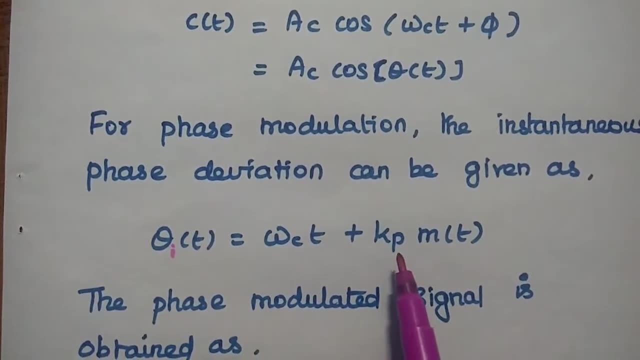 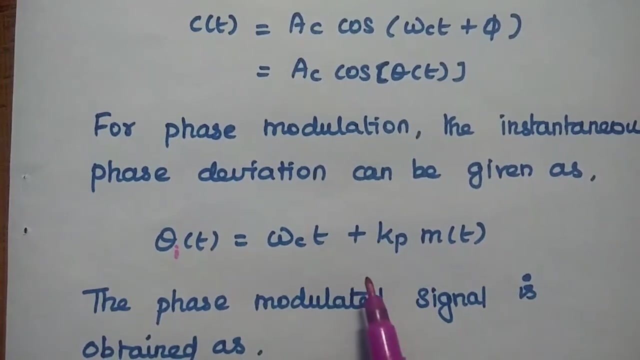 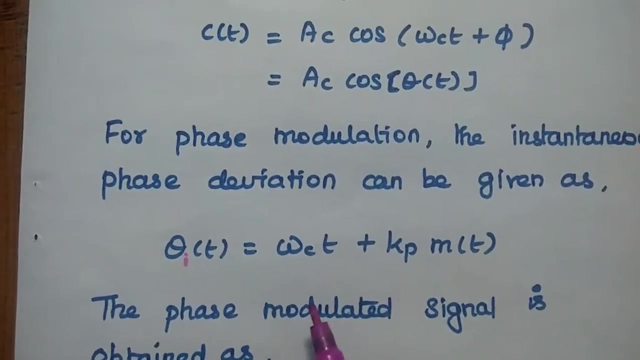 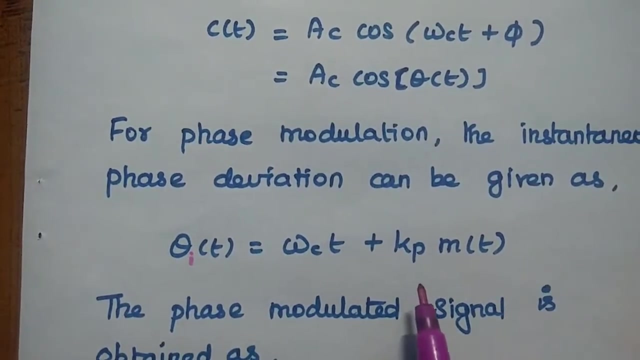 Theta i of t is equal to omega c t plus k p m of t. Here this k? p is nothing but phase sensitivity. So this phase sensitivity actually relates the input and output transfer functions in the modulation process, Because in modulation we are giving the modulating signal which will be modulated into the suitable form using carrier signal. 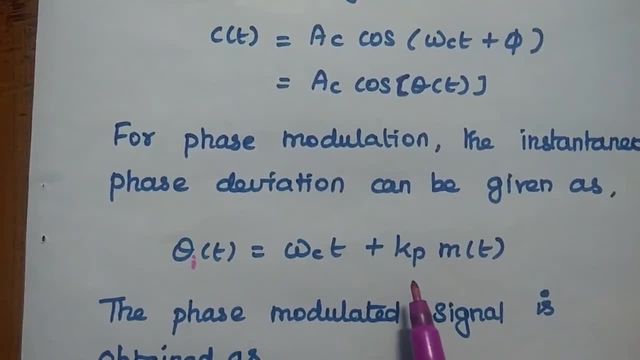 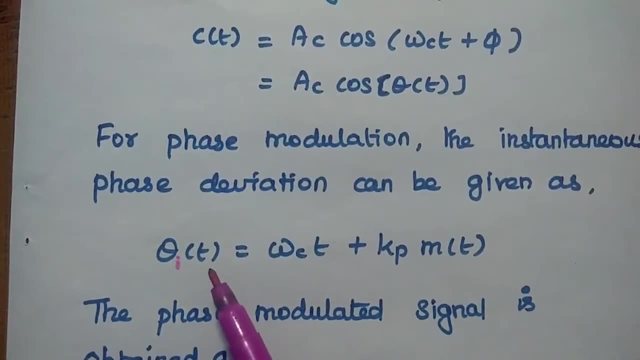 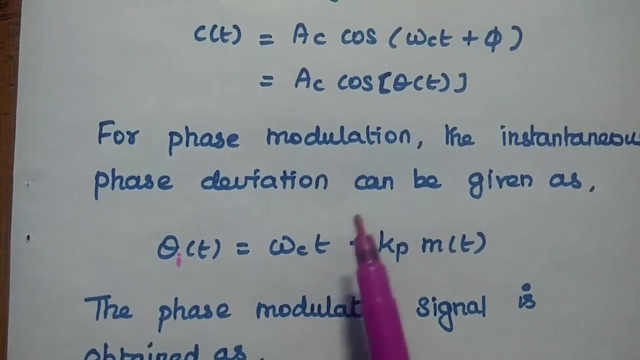 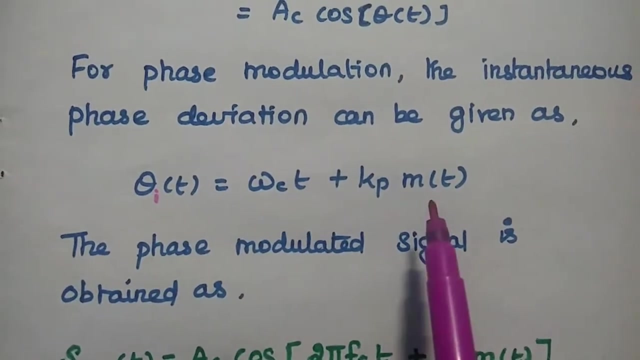 So here this k p represents the phase sensitivity of the modulation process. So the instantaneous phase deviation is nothing but the phase change with respect to the reference phase value of the carrier signal. So here the instantaneous phase deviation depends on the message signal m of t and phase sensitivity. 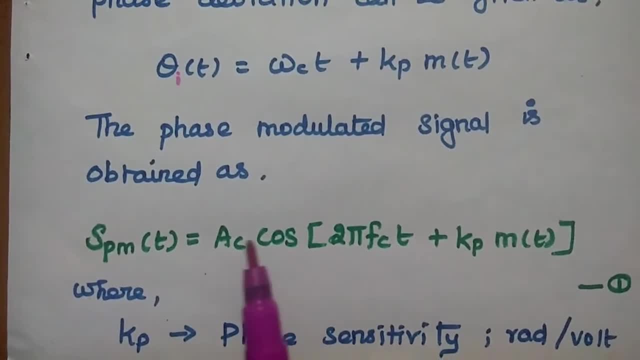 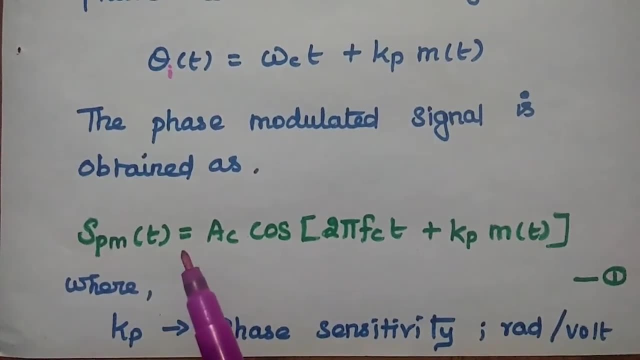 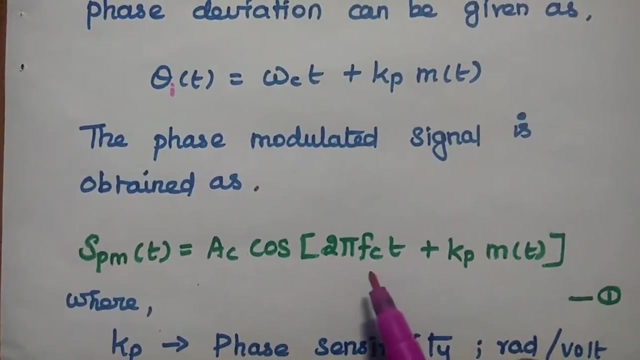 Finally, the phase modulated signal is obtained as s p m of t. Here p m represents the phase modulated signal. So s p m of t is equal to a c cos of 2, pi, f, c, t, that is omega c, t. 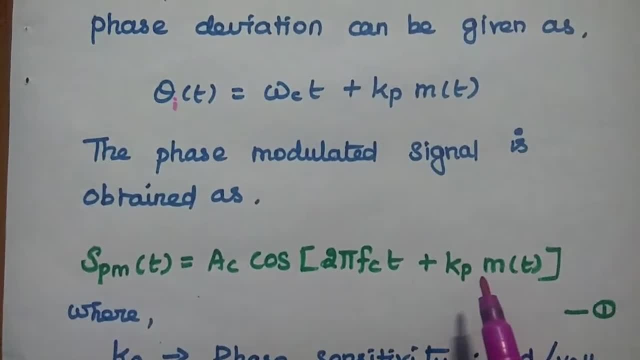 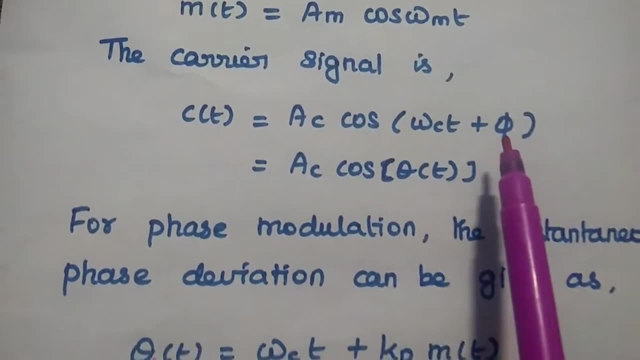 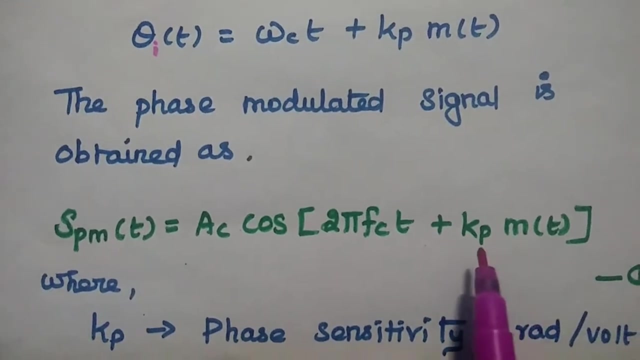 Thus the phase of the carrier signal is changed. Here it is the carrier signal. Actual carrier signal is what a, c, cos of omega c, t plus 5.. So here this phase can be changed. So with respect to instantaneous phase deviation given like k, p, m of t, 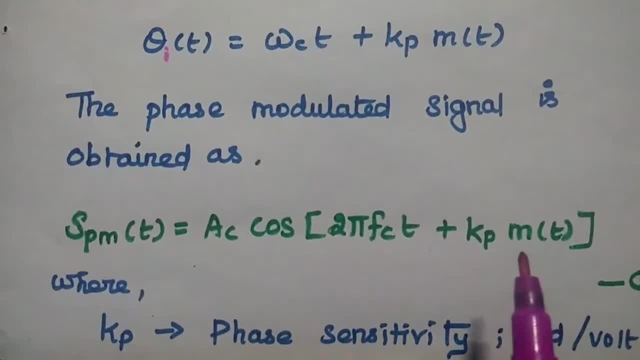 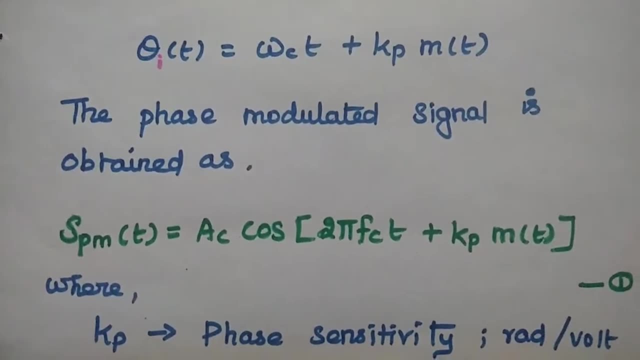 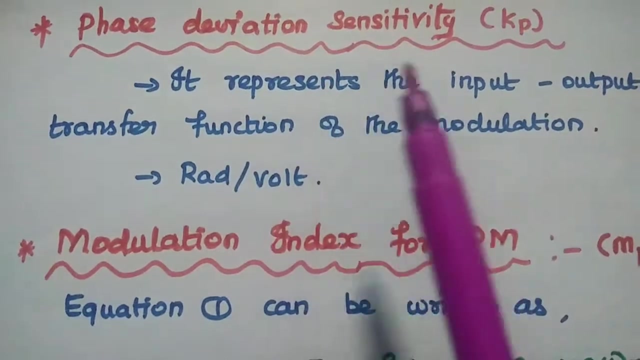 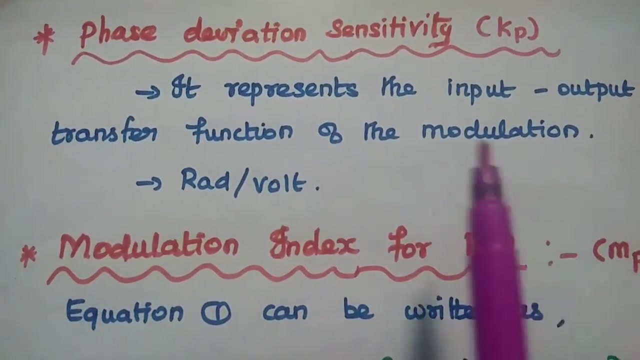 So this is the phase modulated signal. So this k p is measured In terms of radian per volt. Consider this as the first equation. As I told you, phase deviation sensitivity represents the input output transfer function of the modulation process. So here it is measured in terms of radian per volt. 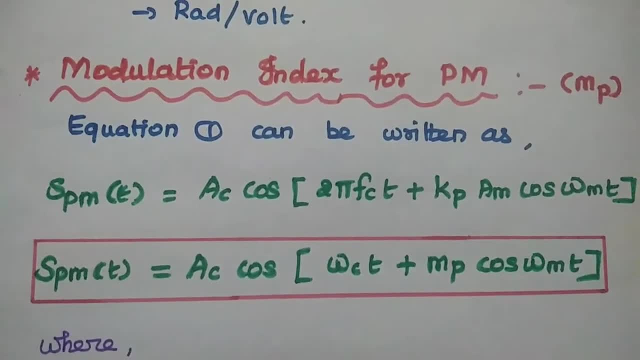 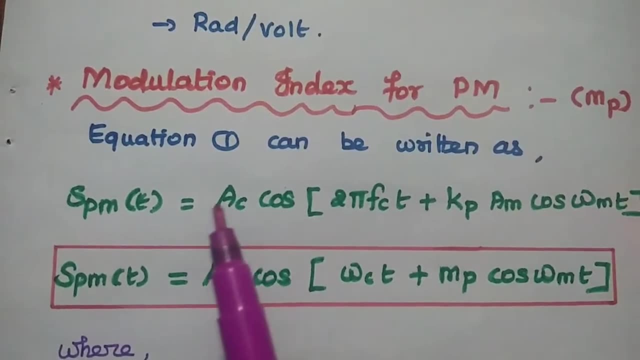 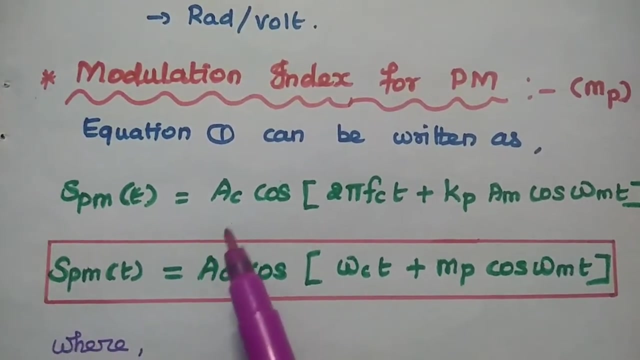 So next we are going to discuss here about modulation index for phase modulation. So simply it is denoted as m suffix p. So here we are going to rewrite the equation 1 as s p, m of t is equal to a, c cos of 2, pi, f, c, t plus k, p. 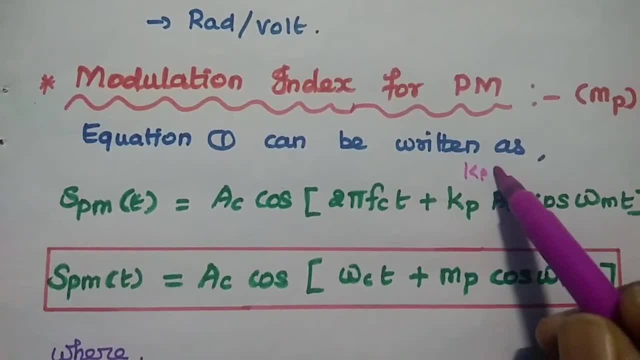 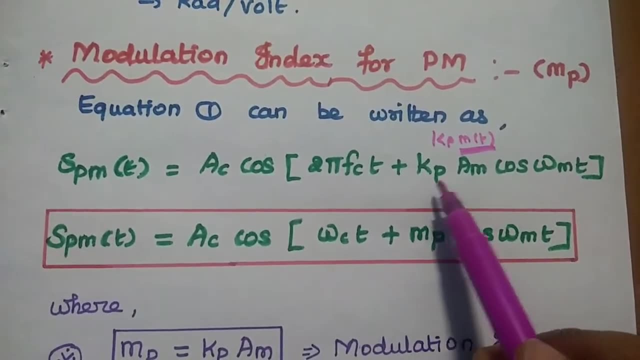 So in the first equation we have written this as k p into m of t, So this m of t is replaced with its expression. So here we can write k p into m of t. is what a, m, cos, omega, m, t. 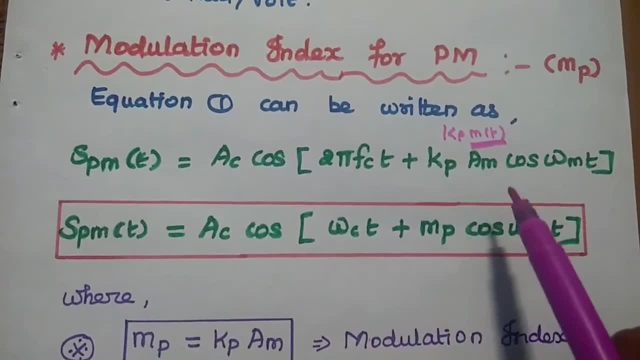 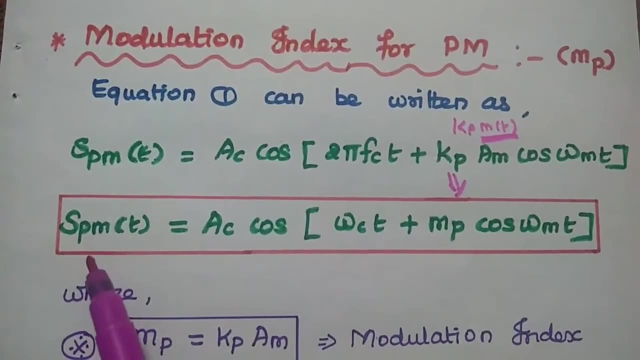 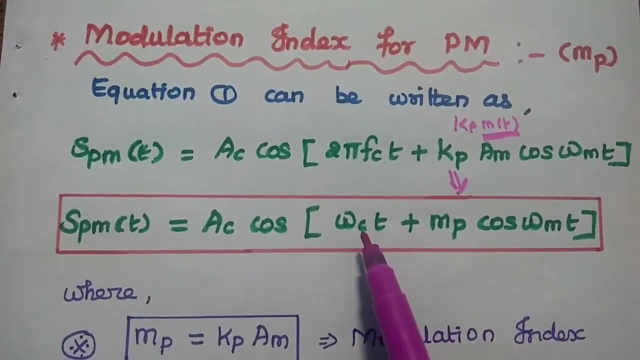 Right, So we can rewrite the expression like this. So now we can simplify this expression as the phase modulated signal s, p, m of t is equal to a c cos of omega c, t, 2, pi f. c means what Omega c, t plus this k, p into a m. 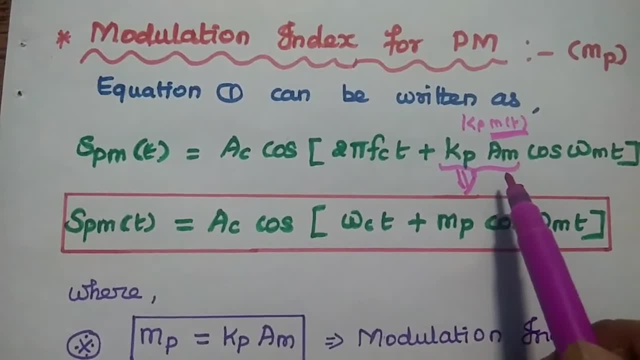 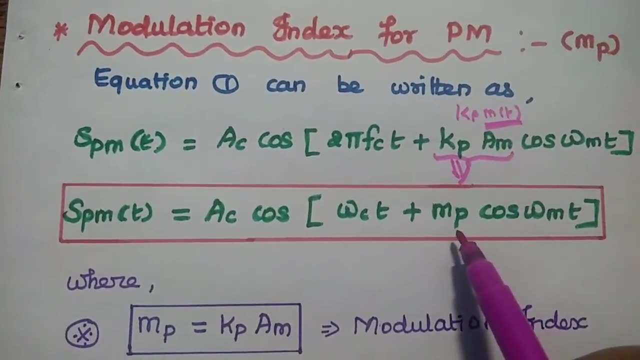 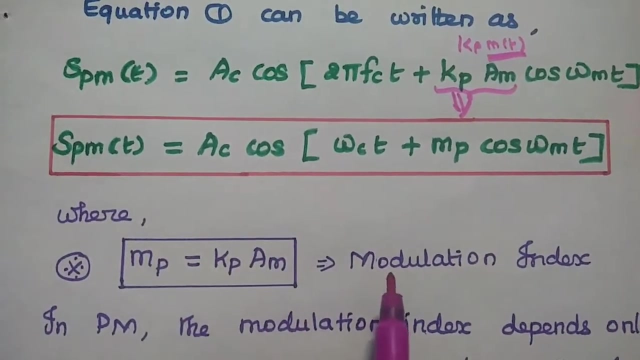 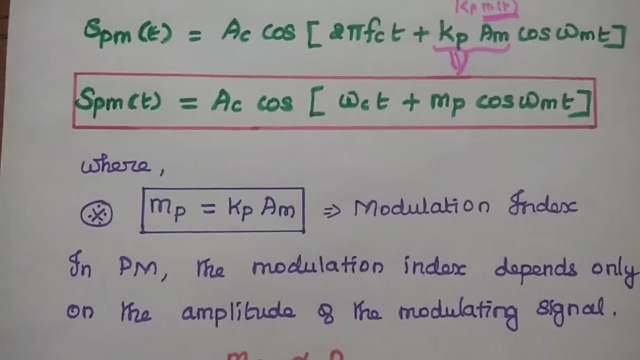 That is the product of phase sensitivity and the amplitude of modulating signal represents the modulation index. So this term becomes m? p and cos omega m t. So here this m p represents the modulation index that is equal to phase sensitivity multiplied with the amplitude of the modulating signal. 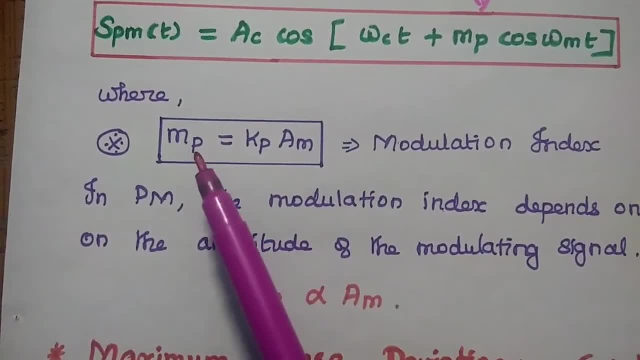 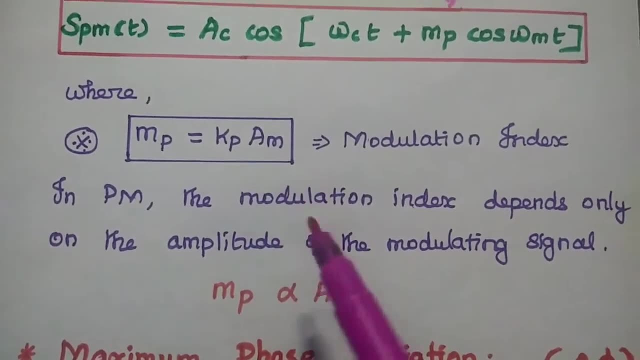 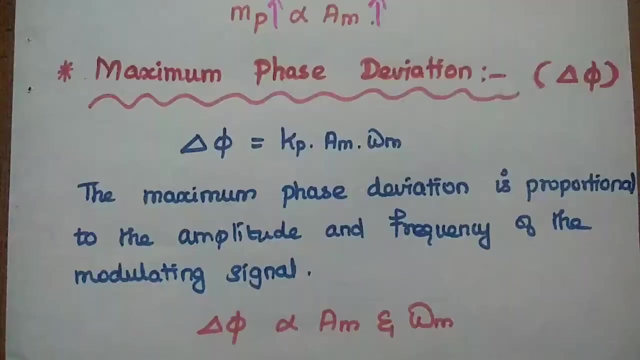 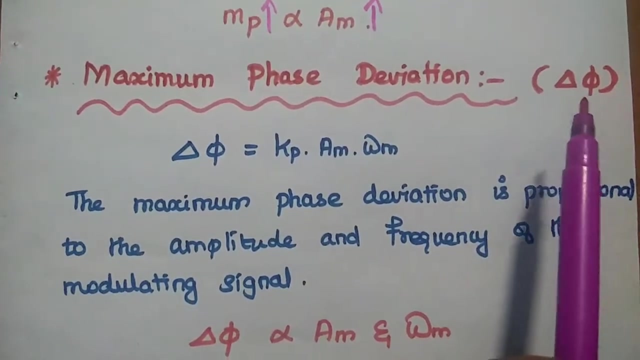 So here in phase modulation the modulation index depends only on the amplitude of the modulating signal. Okay, So if amplitude increases, it increases means its modulation index is also getting increased. So next maximum phase deviation, simply represented as del phi. 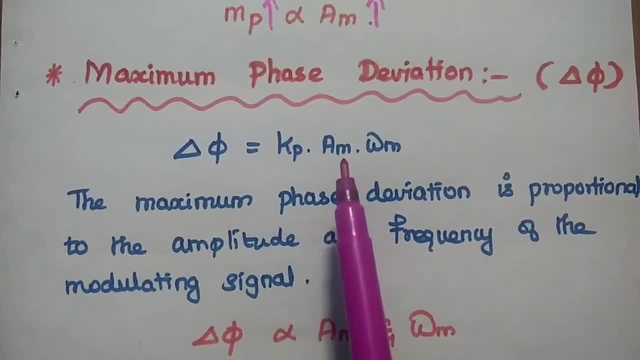 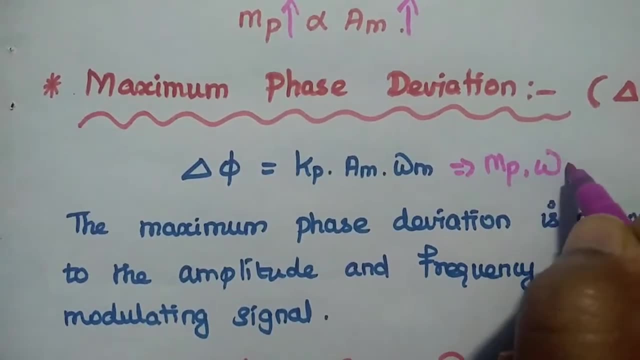 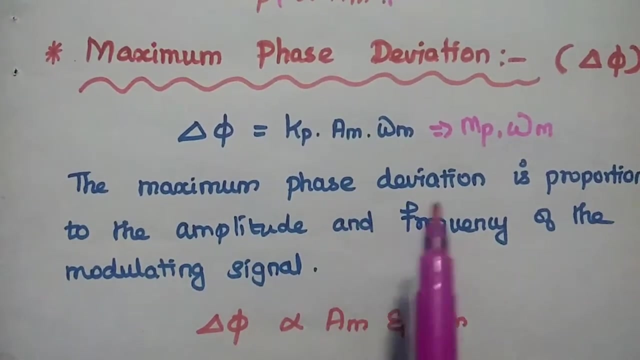 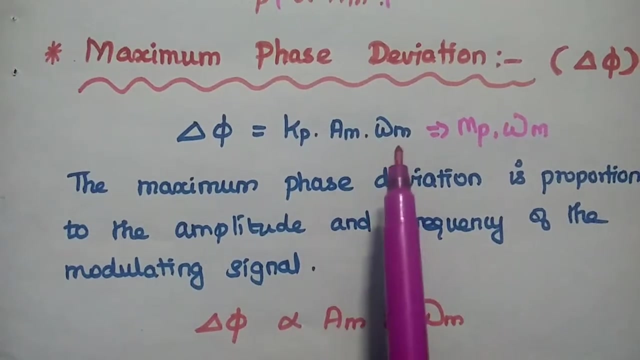 So del phi is equal to k p into a m, into omega m. Simply, we can represent as the modulation index multiplied with the frequency of the modulating signal. Okay, So here the maximum phase deviation is directly proportional to the amplitude as well as the frequency of the modulating signal. 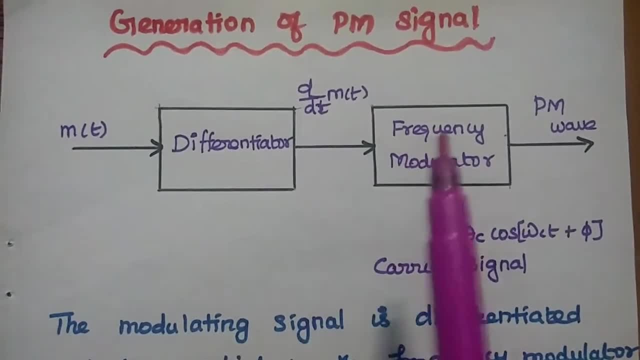 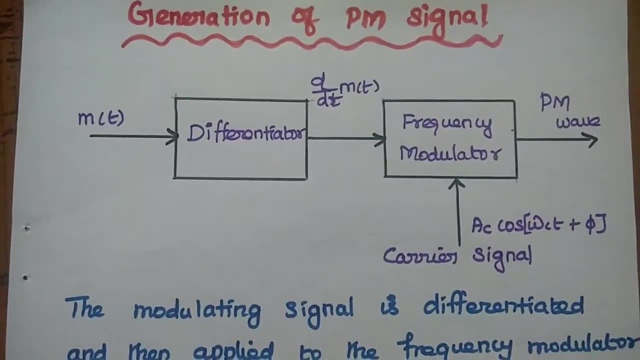 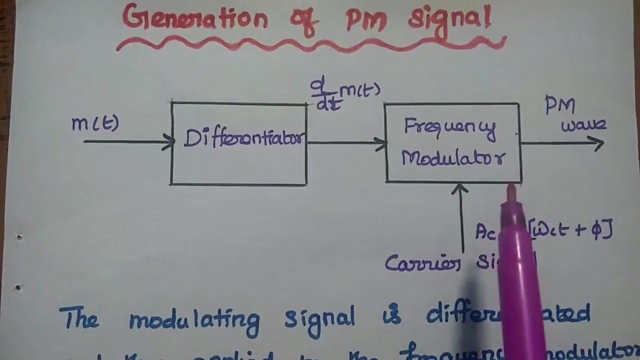 So next, generation of phase modulated signal. So we can generate the phase modulated signal using frequency modulator. So this is the block diagram of generation of p? m signal using frequency modulator. Here we are going to use the differentiator in the first step. 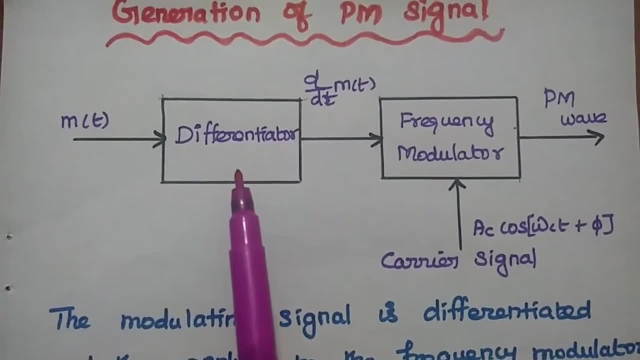 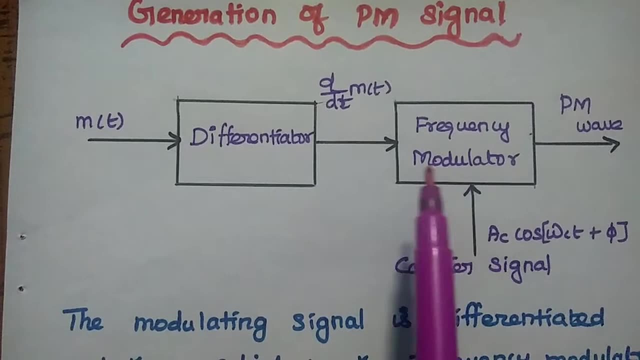 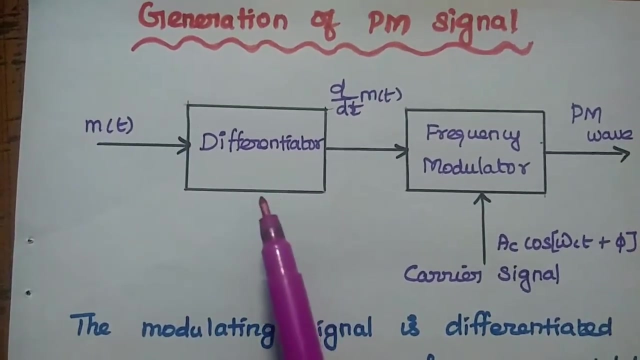 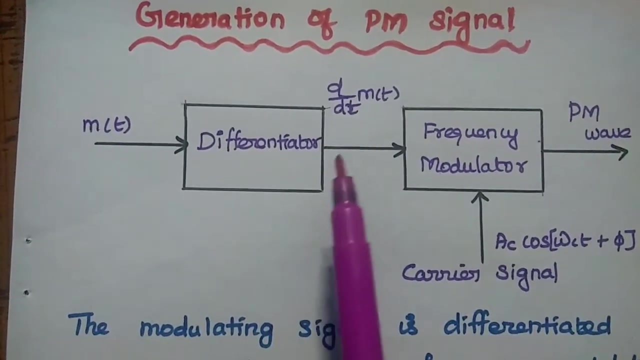 So here the modulating signal is first differentiated and then given as the input to frequency modulator. So for this frequency modulator we need to give the carrier signal also. Okay, So here, why do we need this differentiator? As we know that the differentiation of the phase represents 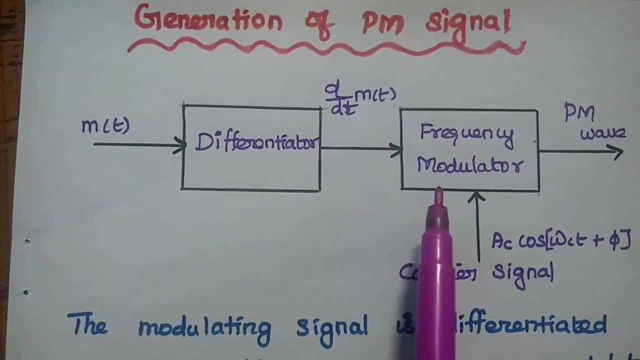 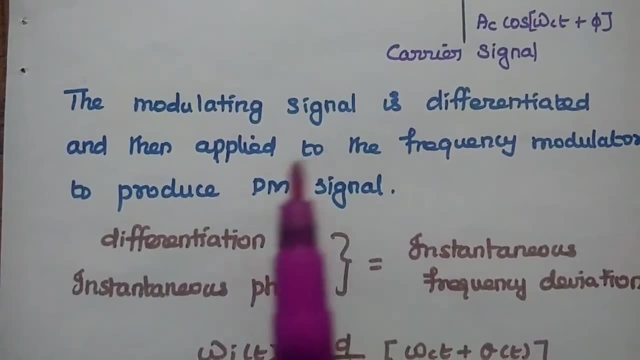 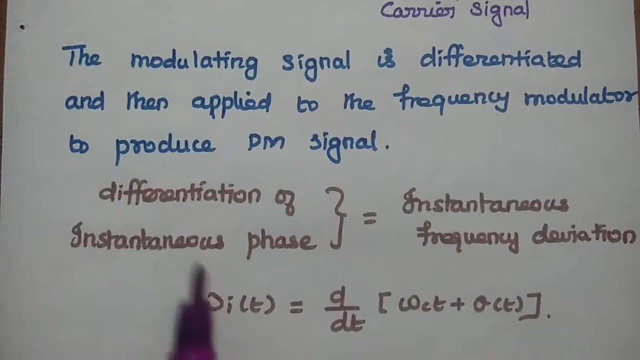 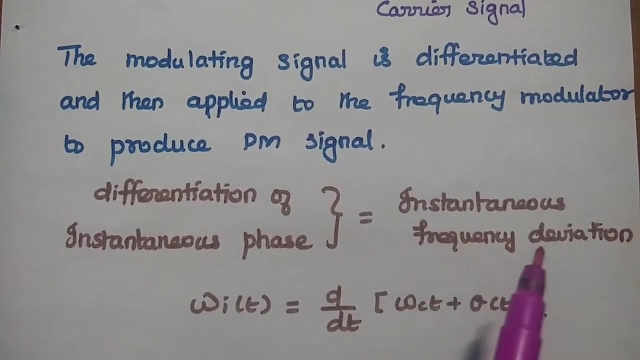 the instantaneous frequency. Okay, So that is the relation over here. That's what given. So the modulating signal is differentiated and then applied to the frequency modulator to produce phase modulated signal. So the differentiation of instantaneous phase is equal to the instantaneous frequency deviation. 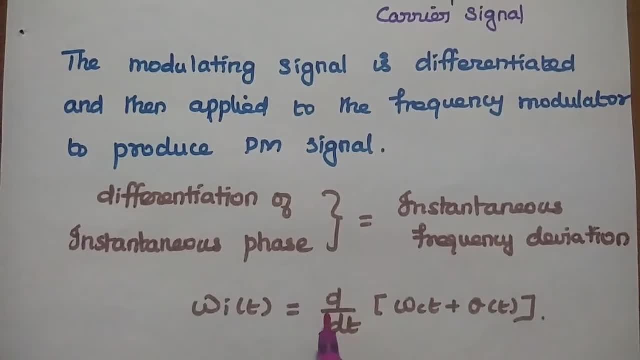 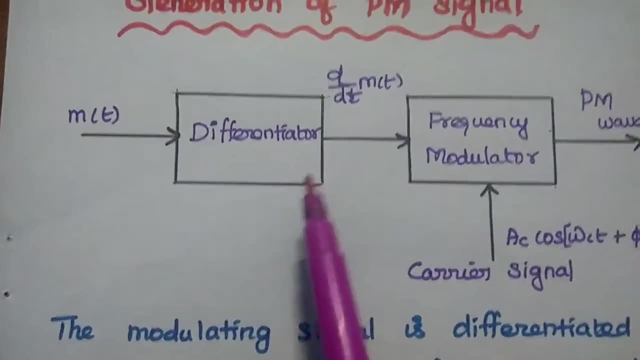 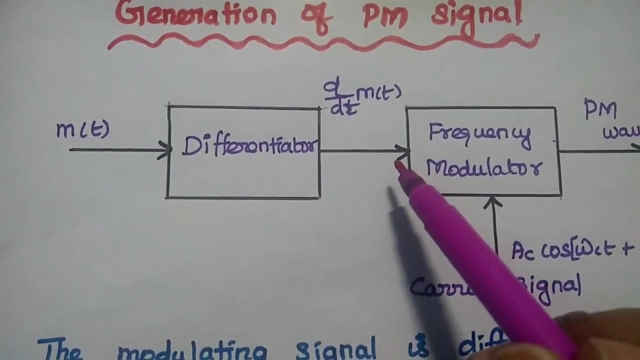 So that's what given here. The instantaneous frequency deviation is equal to d by dt of omega ct plus theta of t. So in this one the signal m of t is differentiated in this differentiator, and then the differentiated value of the phase gives the instantaneous 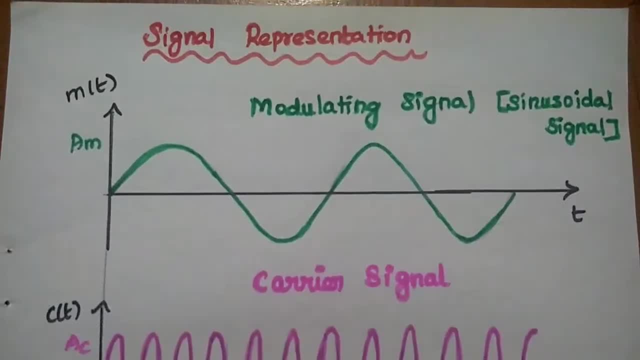 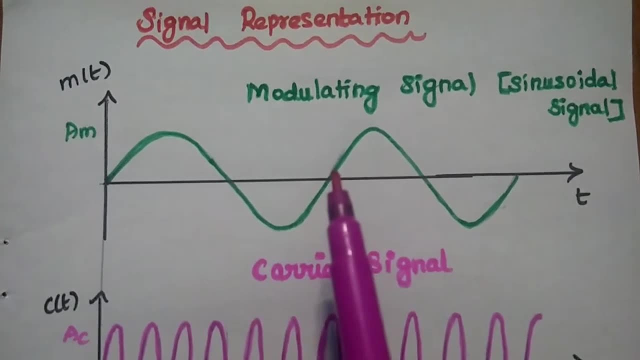 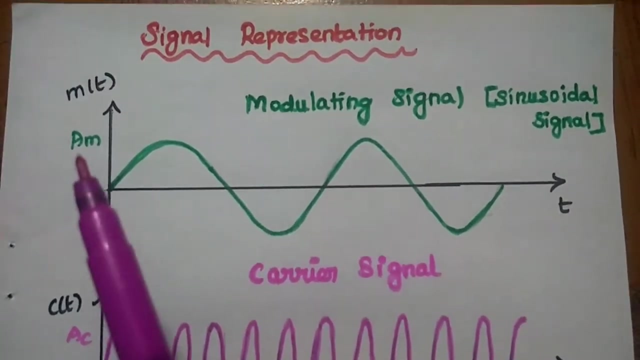 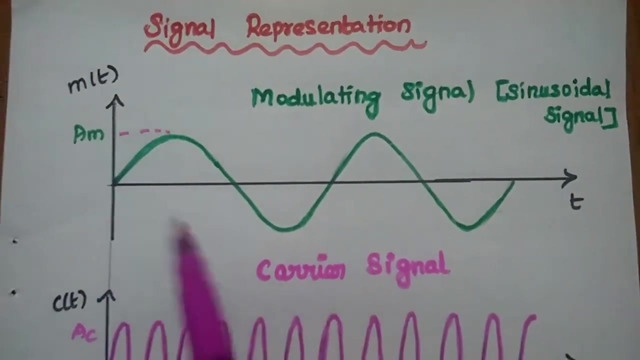 frequency deviation Signal. representation of phase modulated signal. So for that first we have to consider the modulating signal. Here we are considering the sinusoidal signal as a modulating signal that is represented as m of t. So here the maximum amplitude is am. 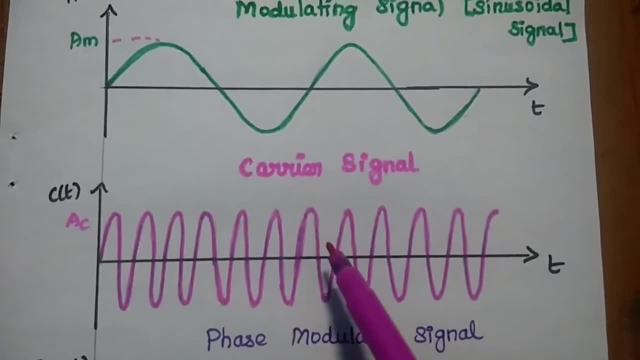 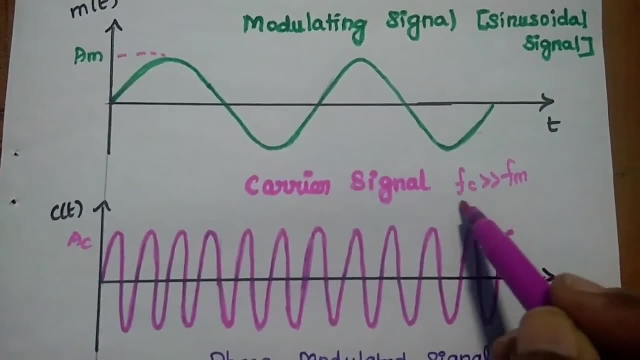 Okay, so the next carrier signal. Carrier signal frequency is always far greater than the modulating frequency. that is the condition here. So we can have the carrier signal line. So we can have the carrier signal line. So we can have the carrier signal line. So 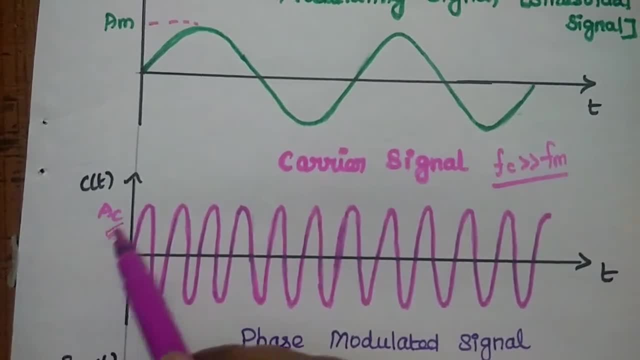 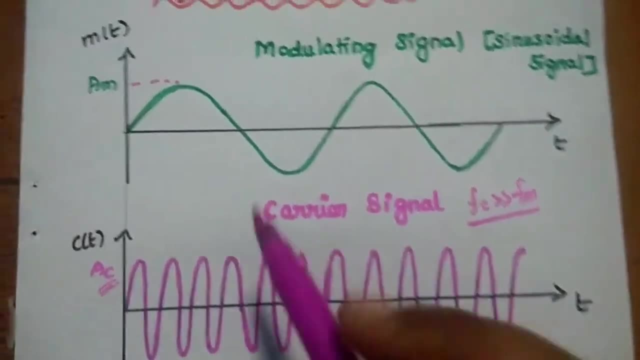 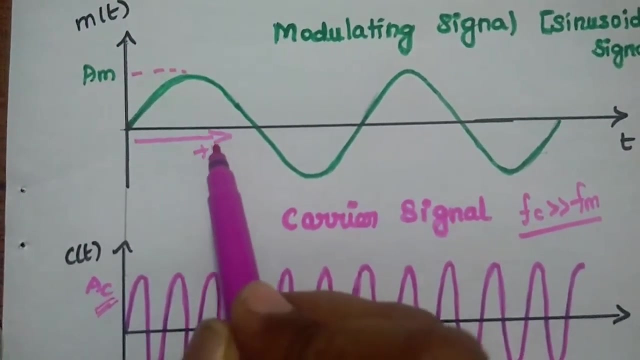 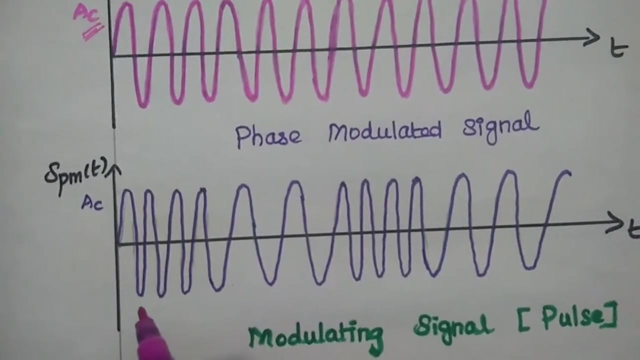 like this and the amplitude of the carrier signal is ac. So next we are going to obtain the phase modulated signal. So here, whenever the amplitude of the modulating frequency is positive, that is, increases, at that time the phase modulated signal phase is leading Okay. 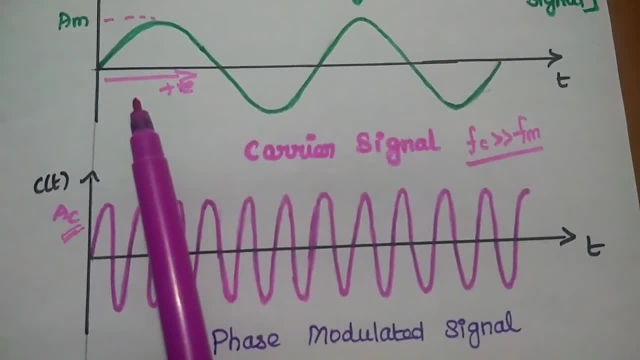 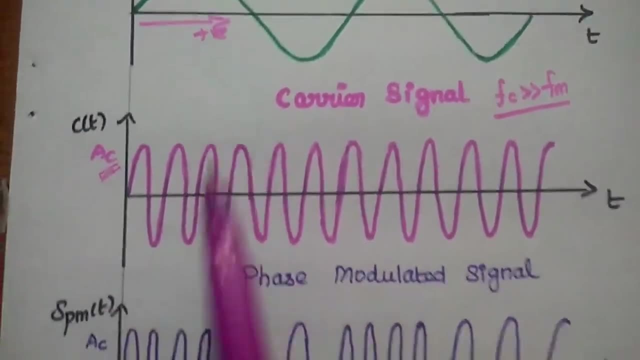 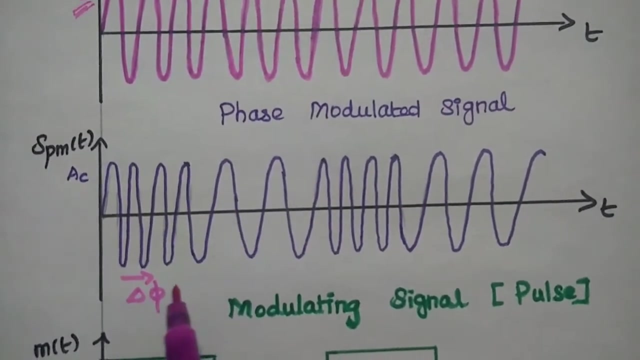 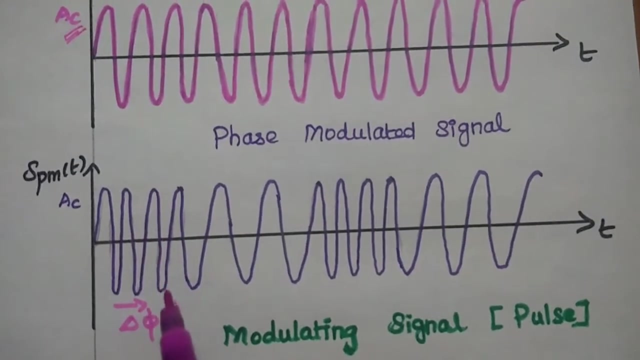 so you have to remember. So whenever The amplitude of the modulating signal is increased, at that time increased as well as positive, at that time the phase deviation, So here the phase deviation of the modulated signal is also increased. So that's why we are having the compressed waveform over here. So here the 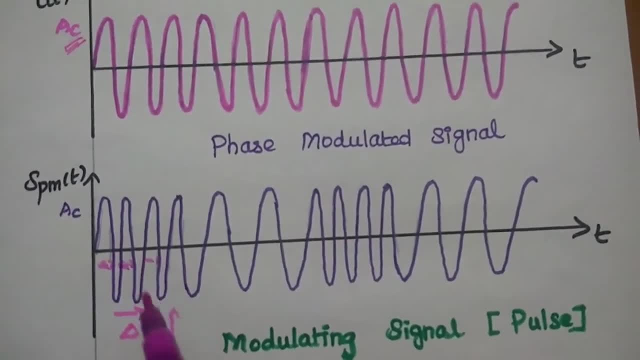 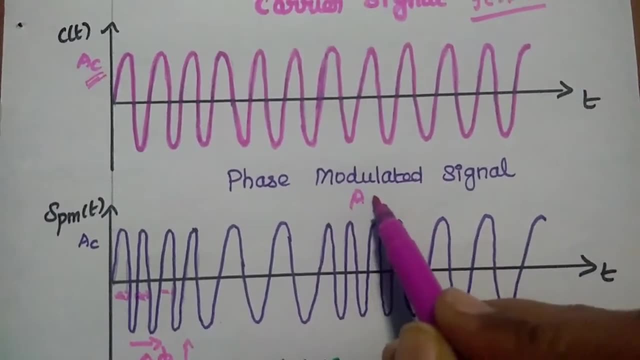 phase. So here the phase is the increased one. Okay, so this is the actual carrier signal. This is the phase modulated signal. So here the phase is the increased one. So this is the actual modulated signal. okay, Phase modulated signal means here AC cos of omega, CT plus KPM of T. 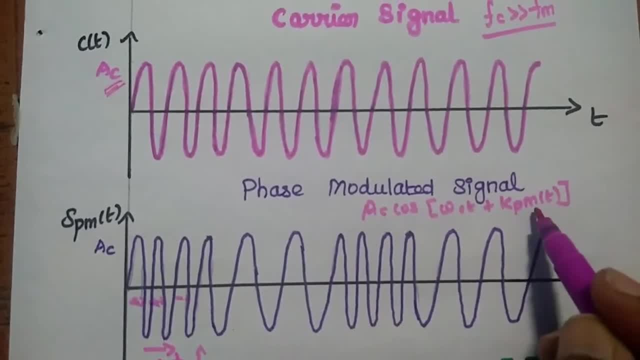 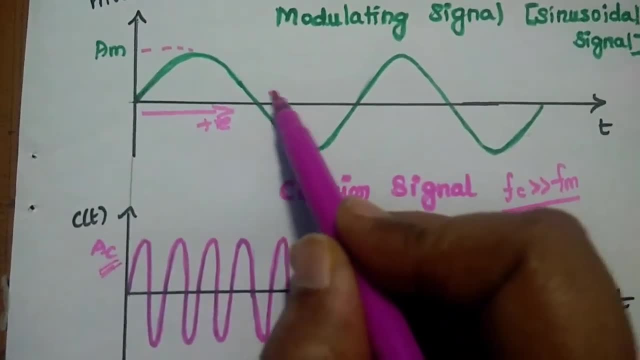 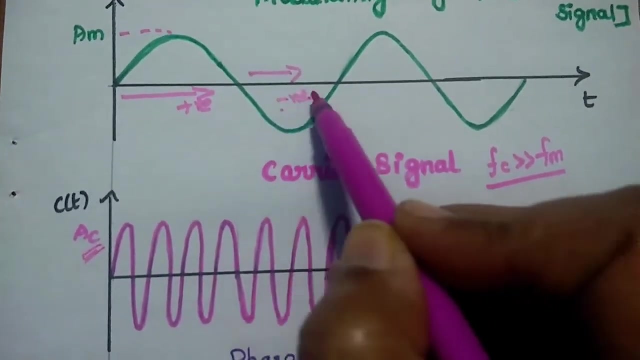 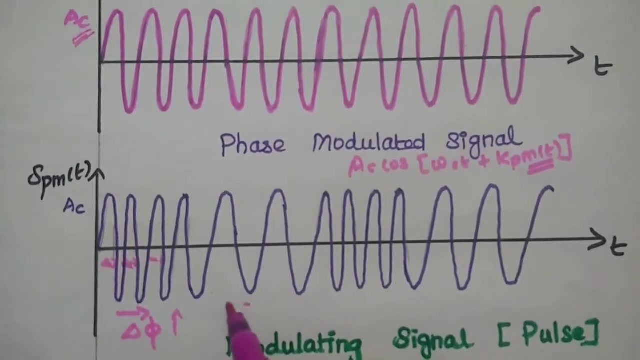 okay, So that is the phase modulated signal, which depends on the modulating signal. okay, So whenever the amplitude of the modulating signal is decreased or in the negative side, okay, At that time the phase deviation of the phase modulated signal lags. That's why. 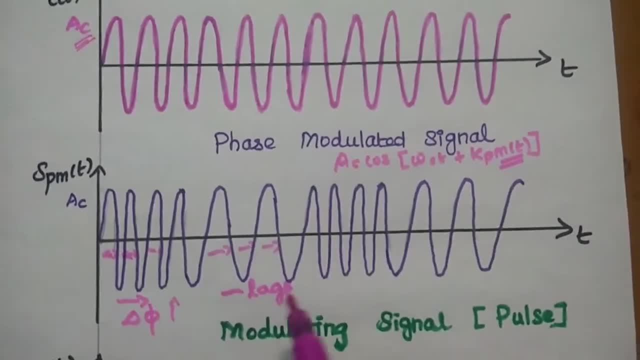 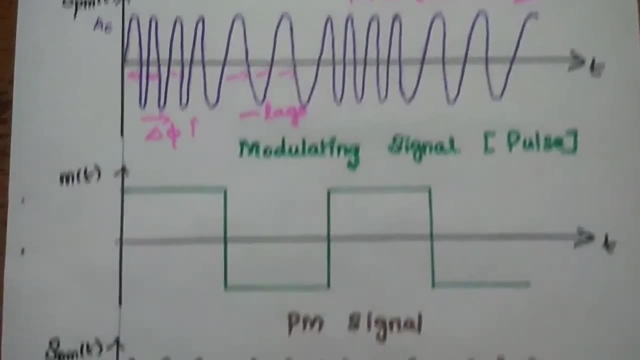 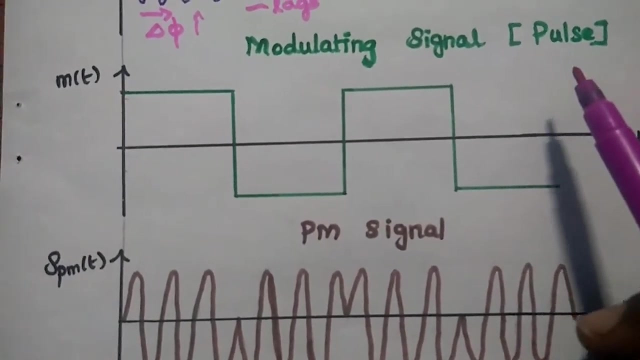 the phases are changed over here. okay, So this is the phase modulated signal for sinusoidal input signal. If I am going to give the modulating signal as a pulse signal, so here pulse signal is a message signal. At that time I can get: 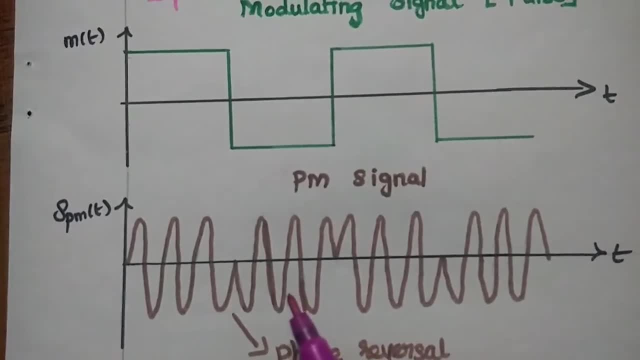 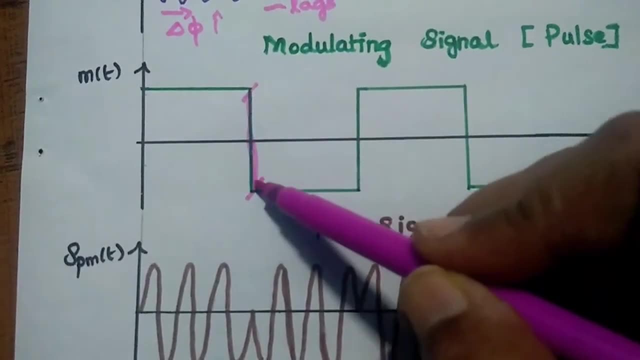 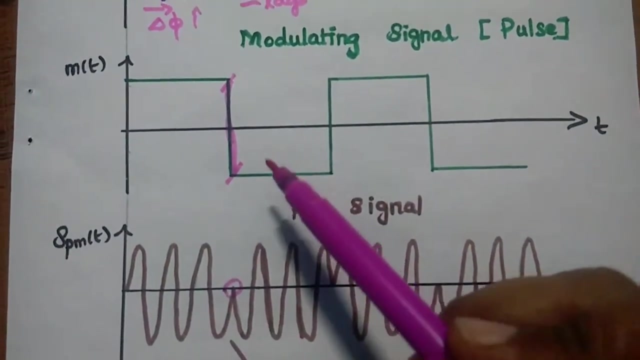 my phase modulated signal like this. So in this case, whenever there is a change from one amplitude to that another amplitude, there is a sudden change, right? So in this condition the phase of the signal is reversed. So whenever there is a change from positive to negative, the signal is 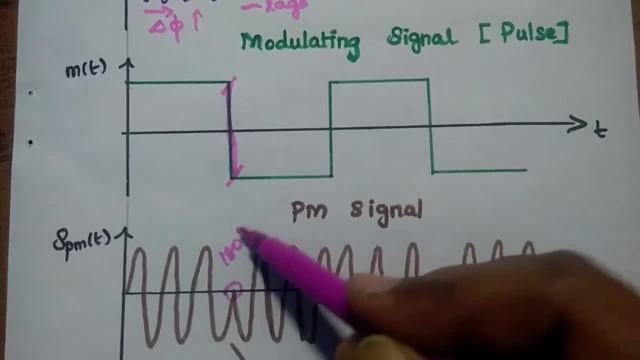 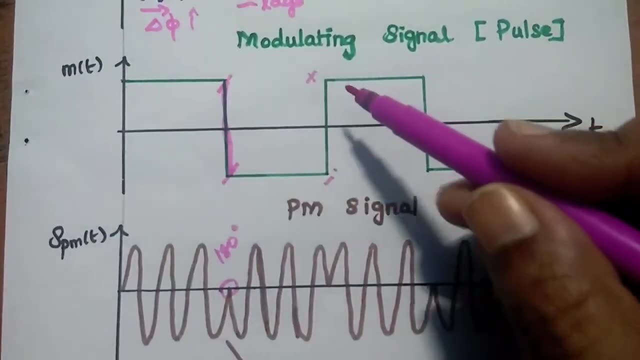 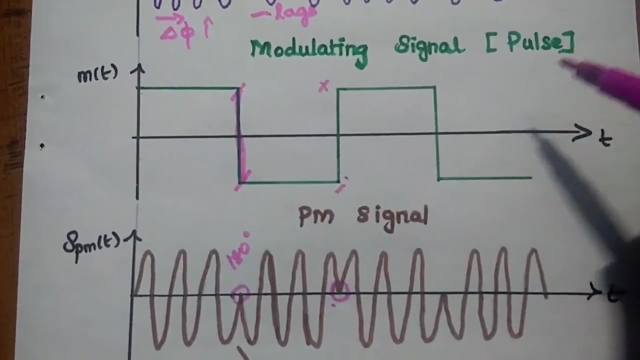 getting reversed 180 degree, okay. So likewise, whenever there is a change from minus to plus, okay, Negative to positive, at that time again there is a phase reversal. So this is the phase modulated signal for pulse signal as input, okay.